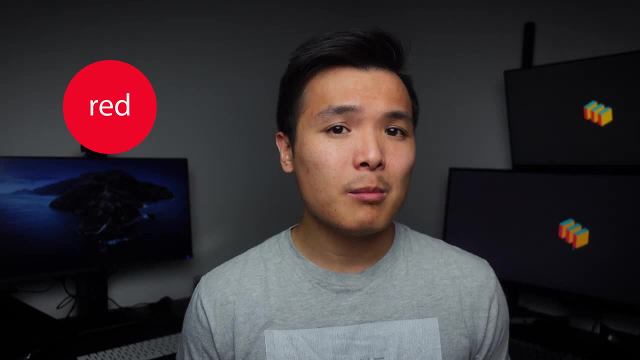 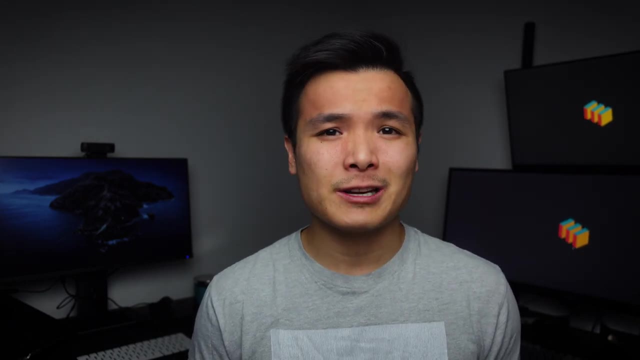 different. Red can be spelled like the color red, but in this context it needs to be spelled like red for reading. So language itself is really complex and it has a lot of nuance and variations that you would have to come up with all possible rules for it as well to have an effective speech. 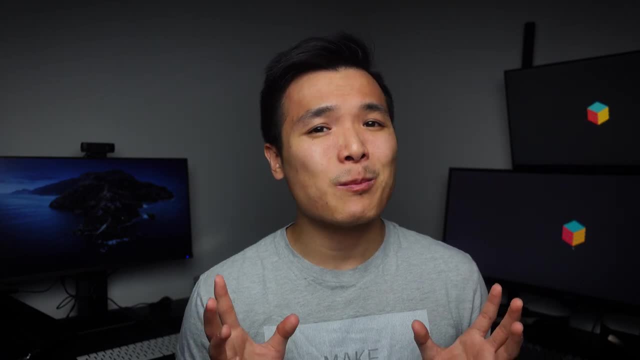 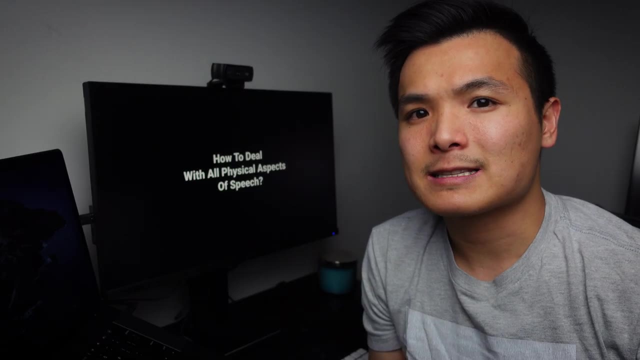 recognition. So what do you do when you have, like, what seems like an insurmountable amount of rules? You use deep learning. So deep learning has changed the game for a lot of complex tasks. Any modern speech recognition system today leverages deep learning in some way. 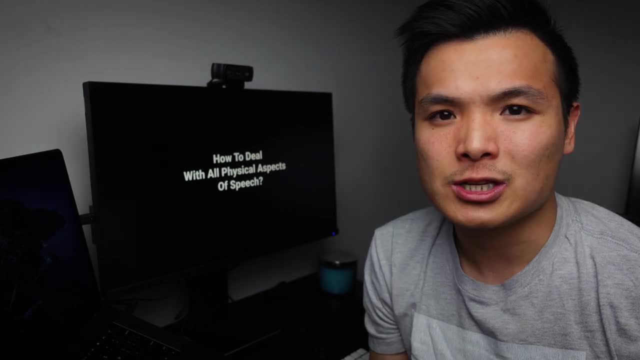 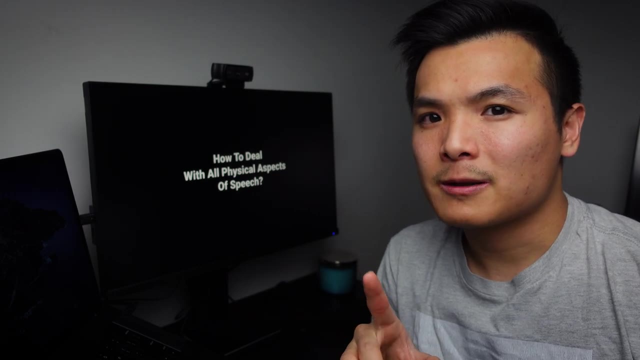 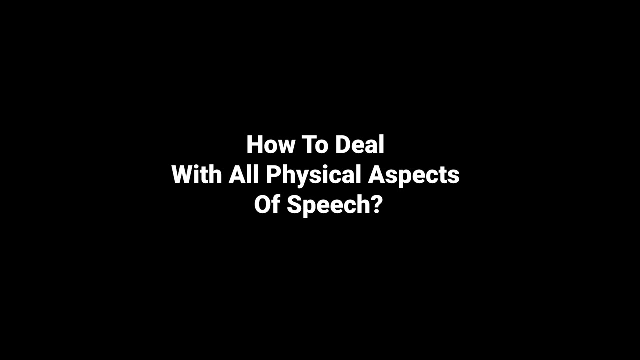 So to build an effective speech recognition system, we have to have a strategy on how to tackle the physical properties of speech as well as the linguistic properties of it. Let's start with the physical property, To properly deal with the variations and nuances that comes with the physicality of speech, like 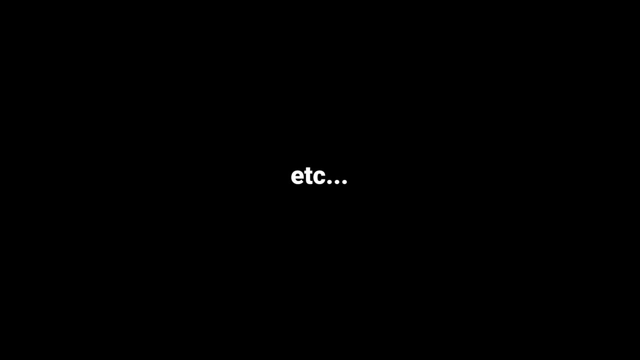 age, gender, microphone, environmental condition, etc. we'll build an acoustic model On a high level. our acoustic model will be a neural network that takes in speech waves as input and outputs to transcribe text In order for our neural network to know how to properly. 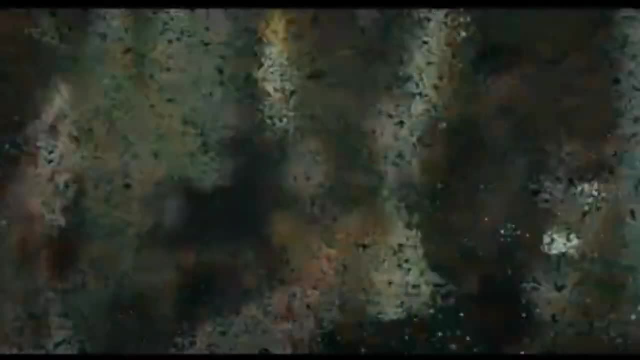 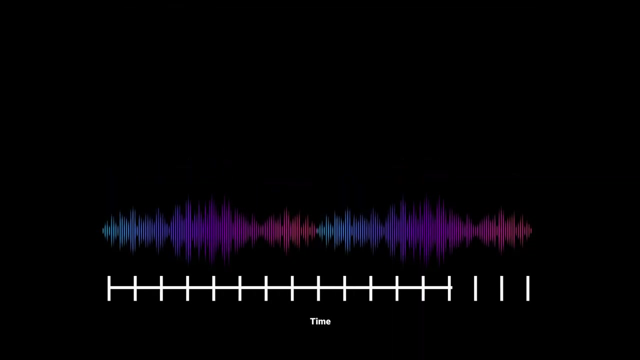 transcribe the speech waves to texts. we'll have to train it with a ton of speech data. Let's first consider what model we want to use by looking at the type of problem we are trying to solve. Speech is a naturally occurring time sequence, meaning we need a neural network that 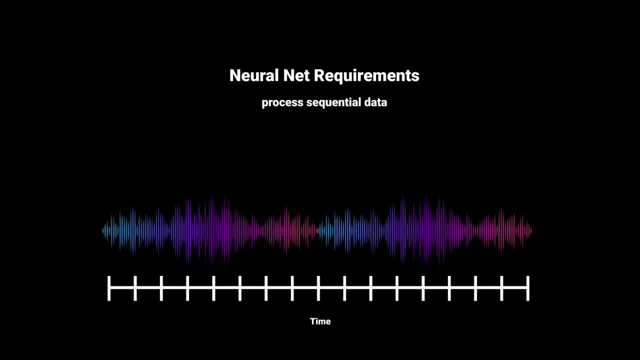 can process sequential data. The neural network also needs to be lightweight in terms of memory and compute because we want to run it real-time on everyday consumer machines. Recurrent neural networks, or RNN for short, are a natural fit for speech recognition. So let's start with the speech. 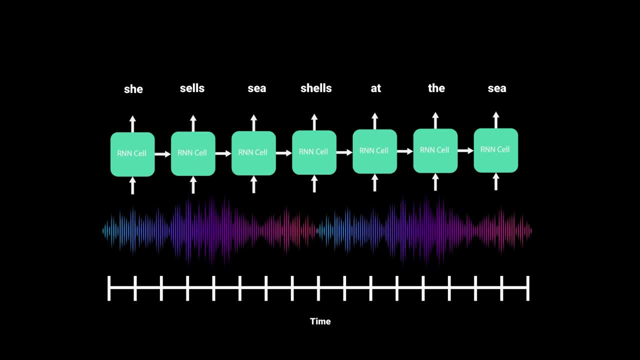 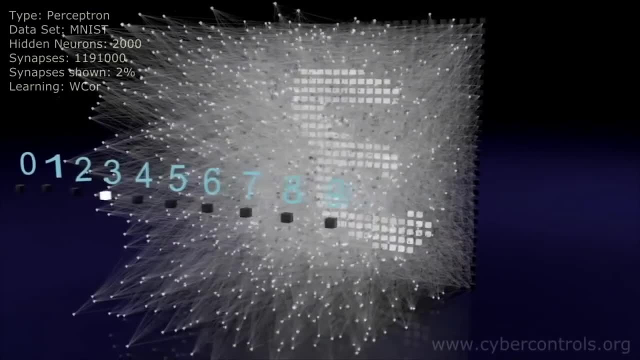 data. The neural network is a neural network that can process sequential data, even when we configure it to be a smaller network size, So we'll use that as our acoustic model. Now let's consider the data. What a neural network can learn is dependent on the data. 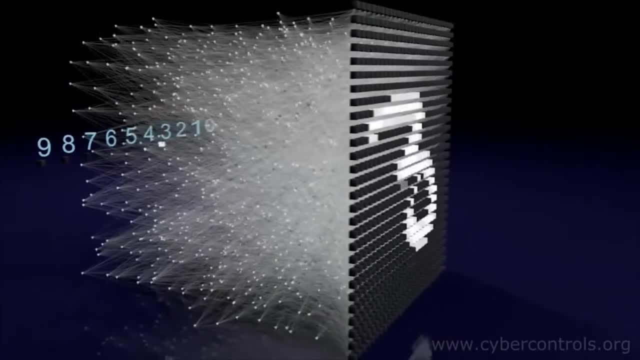 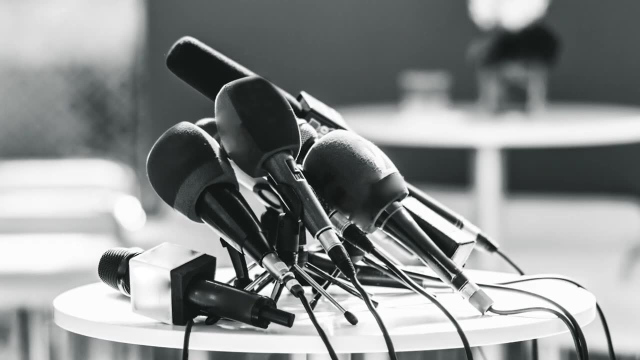 you train it with. If we want our neural network to learn the nuances of speech, we'll need speech data that has a lot of variations of gender, age, accent, environmental noise and types of microphones. Common Voice is an open-source speech dataset. 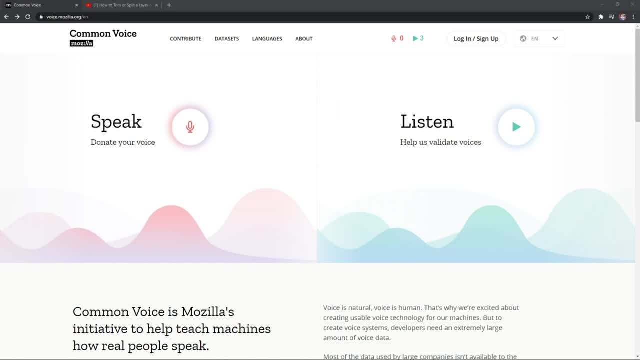 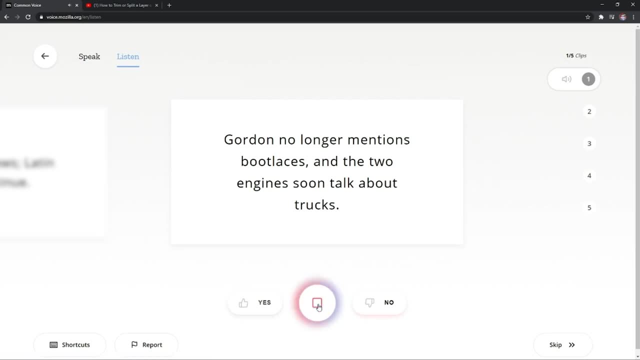 led by Mozilla that has many of those variations, so it'll be perfect. Let's listen to a couple samples. Gordon no longer mentions bootlaces and the two engines soon talk about trucks. Faith is granted Jews. Latin colonies continue. It has since been renamed Yersin Arafat International Airport. 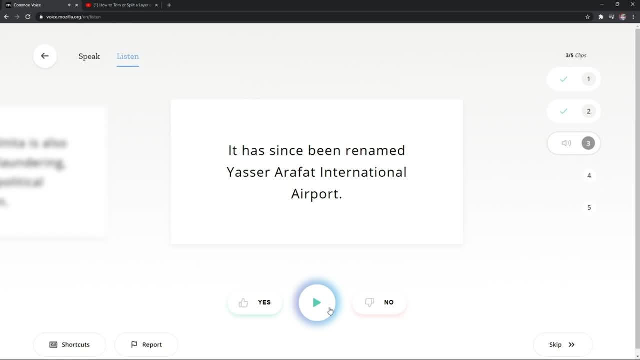 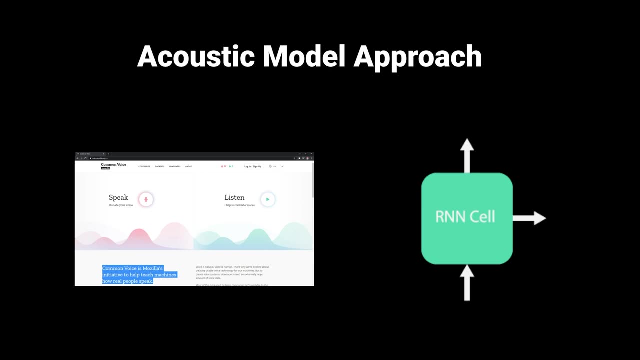 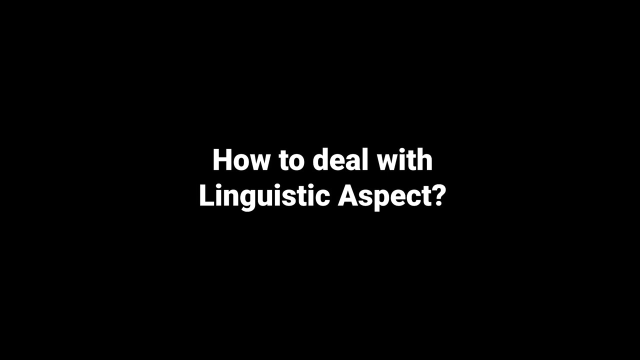 Each audio sample comes with labels of the transcribed text. Okay, I think we have a solid approach. We have a dataset that contains some variation in nuances, as well as a lightweight neural network architecture. Now let's talk about the linguistic aspect of speech. To inject linguistic features into the 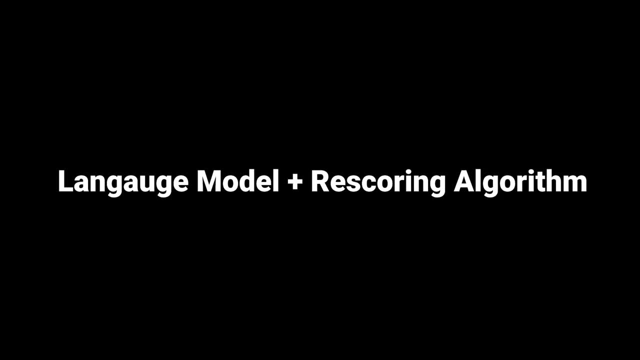 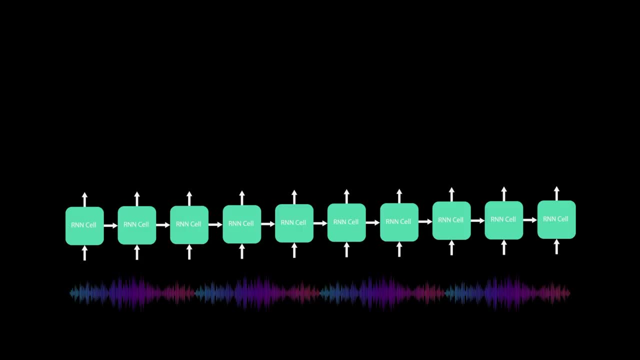 transcriptions. we'll use something called a language model alongside a rescoring algorithm. To understand how this works at a high level, let's look at the acoustic model's output. A speech recognition neural network is probabilistic, so for each time step it outputs a probability. 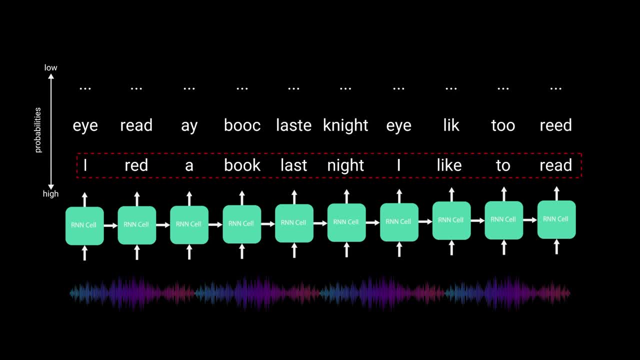 of possible words. You can naively take the highest probable word of each time step and emit that as your transcript, but your network can easily make linguistic mistakes, like using the word red for color when it should be red for reading. This is when the language model comes into play. 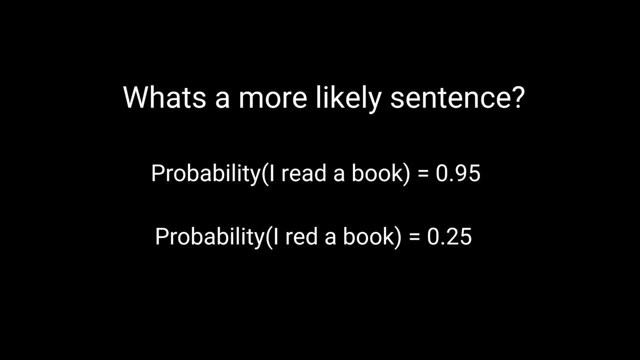 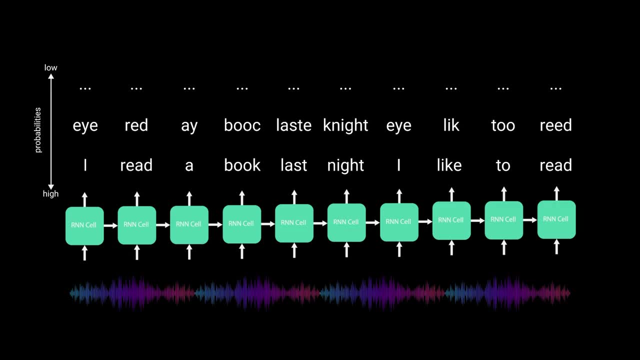 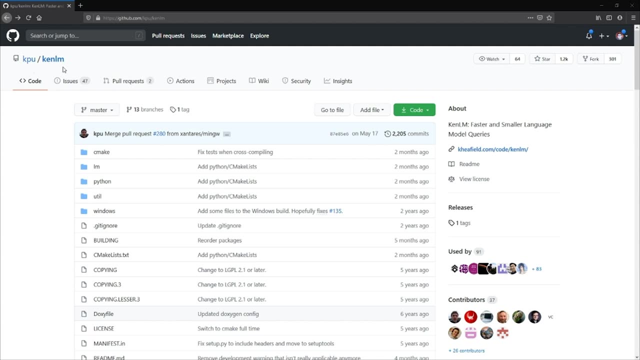 A language model can determine what is a more likely sentence by building a probability. You can use a language model and rescore the probabilities depending on the context of the sentence. You'll get an idea of how all this works in a minute. For our implementation of a language model, we can use an open source project called KenLM, which is a rules-based language model. 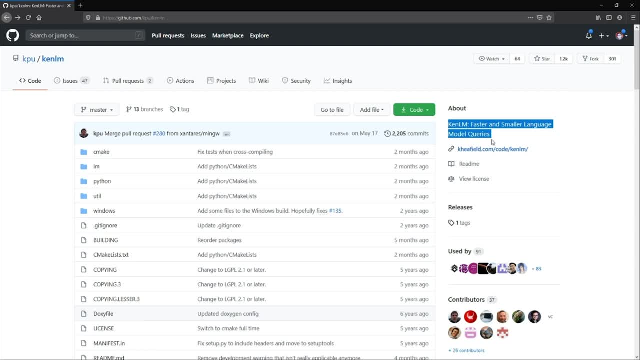 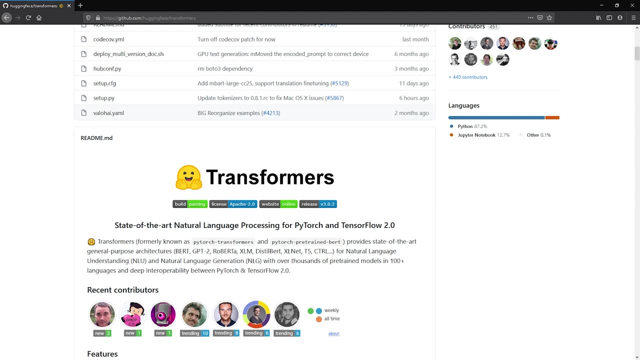 We want to use KenLM because it's lightweight and super fast, unlike the much heavier neural network-based language models. A neural-based language model, like Transformers from Hugging Face, have been proven to produce better results, but since our goal is low compute, we'll use KenLM, which works well enough. 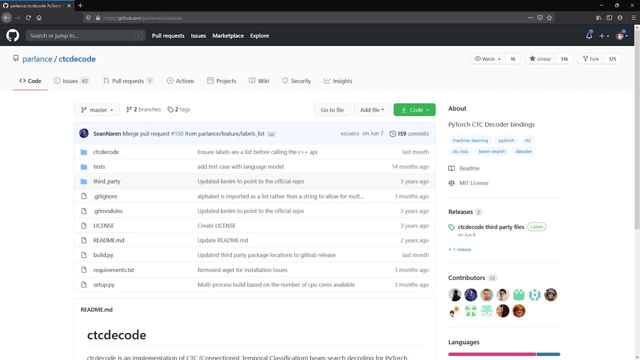 For the rescoring algorithm, we'll use what's called a CTC beam search. The beam search combined with the language model is how we'll rescore the outputs for better transcriptions. The logic of the beam search algorithm can get pretty complex and very boring. 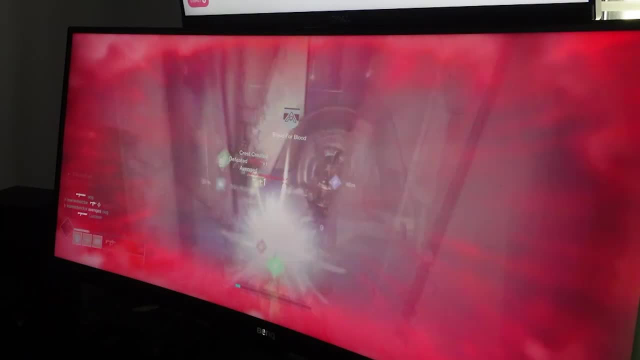 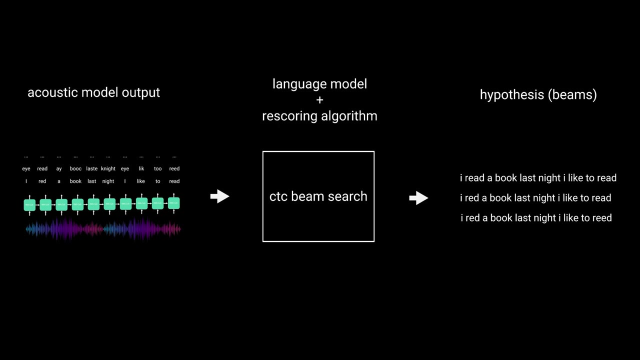 and I'm way too busy to attempt an in-depth explanation here, but here's the basic premise: The beam search algorithm will traverse the outputs of the acoustic model and use the language model. We'll use the language model to build hypotheses, aka beams, for the final output. 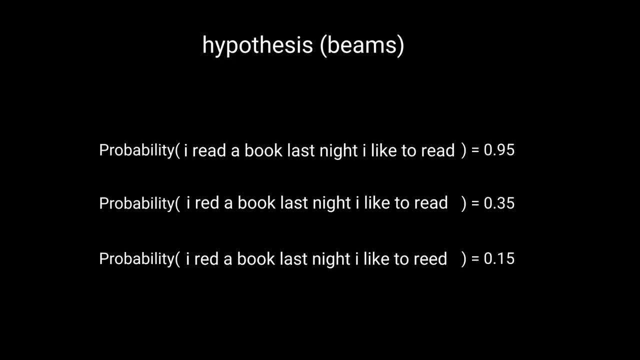 During the beam search. if the language model sees that the word book exists in the transcription, it'll boost the probability of the beams that contains red like reading instead of red like color, because it makes more sense. This process will produce more accurate transcriptions. 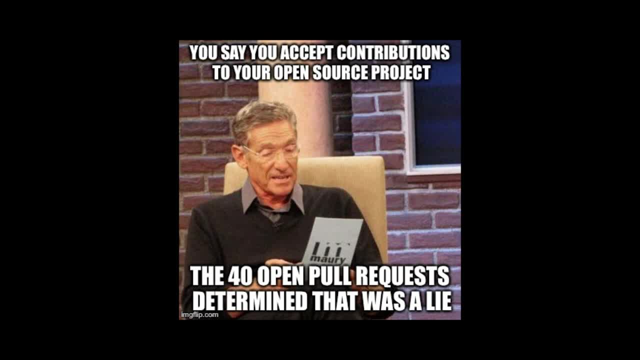 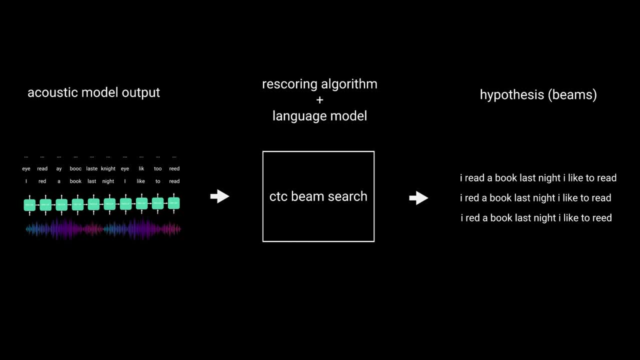 Thank the programming guides for open source code, so we don't have to build the language model and the CTC beam search rescoring algorithm ourselves, which will save us a ton of time. So, to sum it up, using a language model and a CTC beam search algorithm. 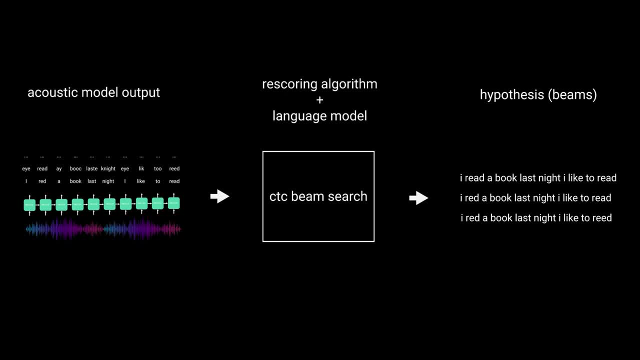 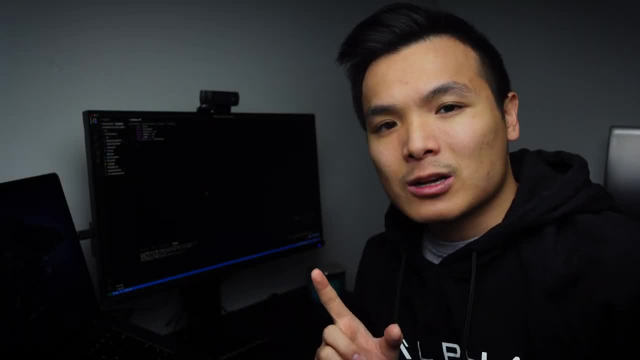 we can inject language information into the acoustic model's output, which results in more accurate transcriptions. Okay, I think we have a pretty solid strategy on how to tackle this speech recognition problem. For the physical properties, we'll implement an acoustic model. 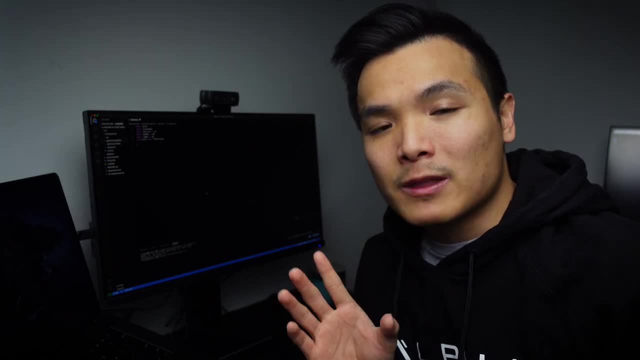 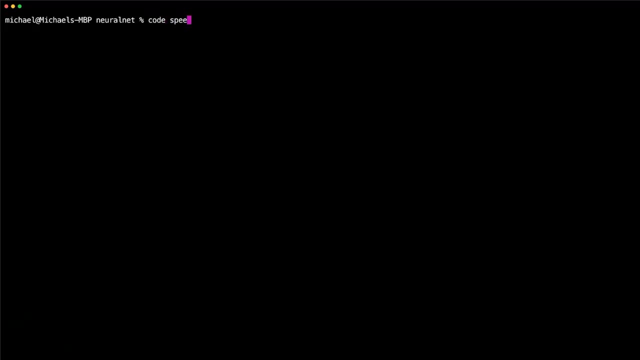 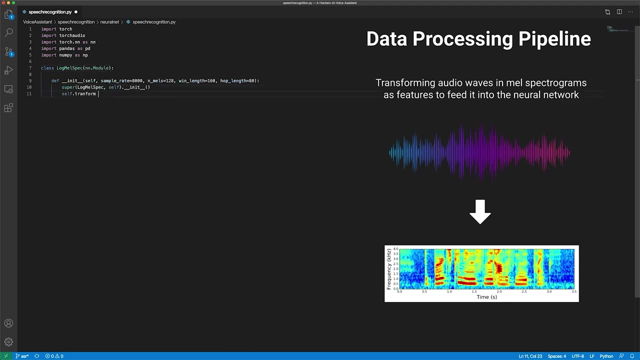 and for the linguistic properties, we'll implement a language model with a rescoring algorithm. Let's get to building. First, we need to build a data processing pipeline. We'll need to transform the raw audio waves into what's called MEL spectrograms. 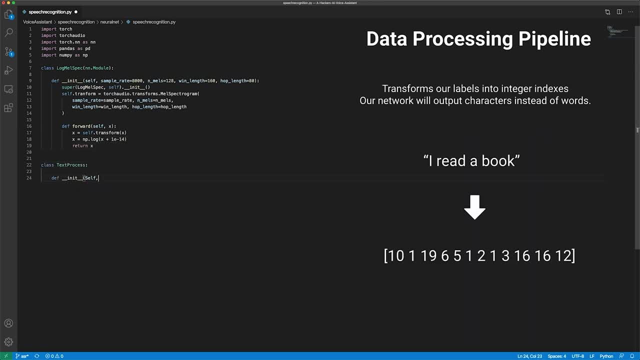 You can just think of MEL spectrograms as a pictorial representation of sound. We'll also need to process our character labels. Our models will be character-based, meaning it will output characters instead of word probabilities. Decoding character probabilities is more efficient. 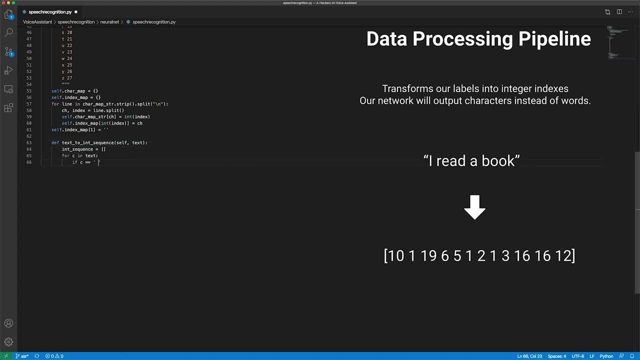 because we won't have to worry about 27 probabilities for each output instead of like 100 or 1000 of possible words. We'll need to augment our data so we can effectively have a bigger data set. We'll use spec augment. Spec augment is augmentation technology. 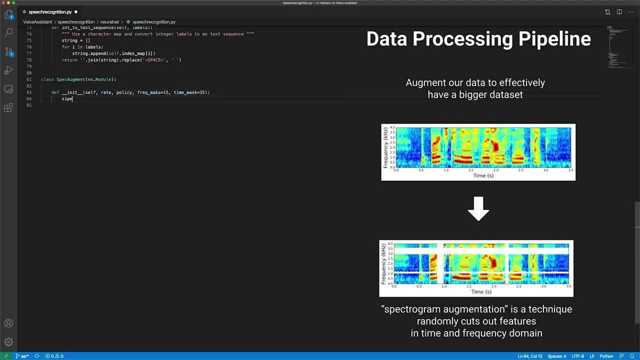 that cuts out the information in the time and frequency domain, effectively destroying pieces of the data. This makes the neural network more robust because it's forced to learn how to make correct predictions with imperfect data, making it more generalizable to real world. 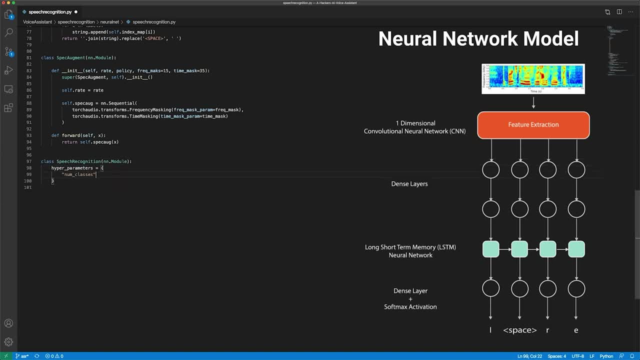 Now let's move on to the model. The model will consist of a convolutional layer, three dense layers and an RNN LSTM layer. The purpose of the convolutional layer is two things: It learns to extract better features from the MEL spectrogram. 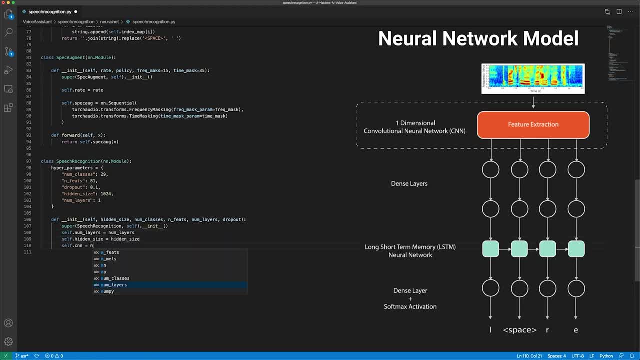 and also reduce the time dimensions of the data. In theory, the CNN layer will produce features that should be more robust, causing the RNNs to produce better predictions. We also set the stride of the CNN layer to be higher, from 1 to 2,. 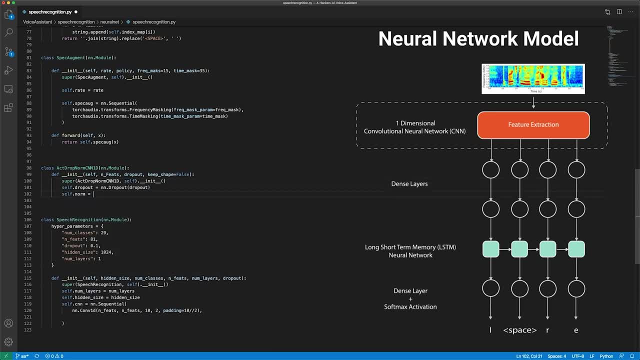 therefore reducing the time steps of the MEL spectrogram by half, allowing the RNNs to do less work because there are less time steps, which would make the overall network faster. We add in two more dense layers in between the CNN and the RNNs. 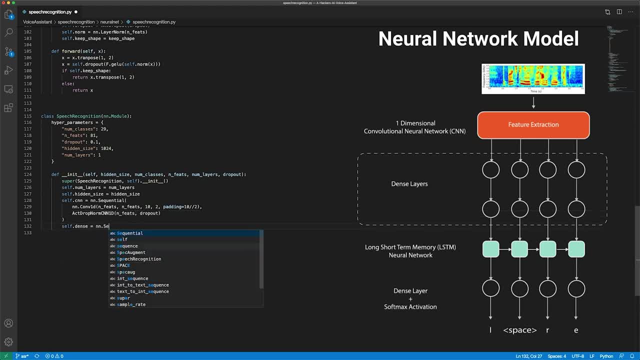 The purpose of the dense layer is to also learn to produce a more robust set of features for the RNNs. For the RNN layer, we used an LSTM variant. The RNN takes the features produced by the previous dense layer and, step by step, produces an output that can be used for prediction. 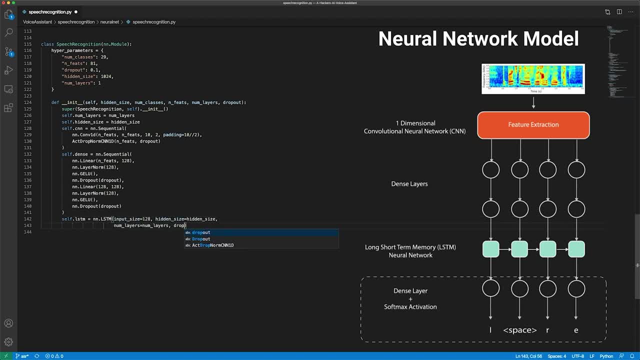 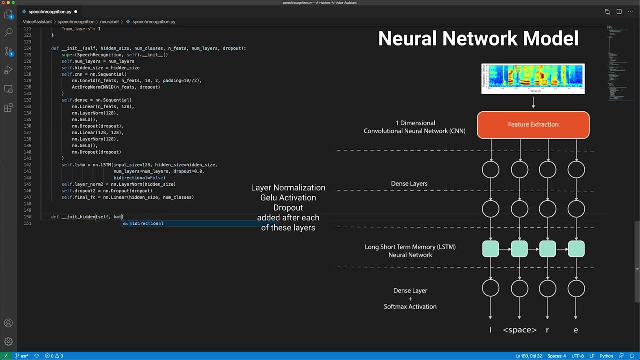 We also have a final dense layer with a softmax activation that acts like a classifier. The classifier takes the RNNs output and predicts character probabilities for each time step. We add layer normalization, GELU activation and dropout between each layer with the purpose of making the network more generalizable and robust to real-world data. 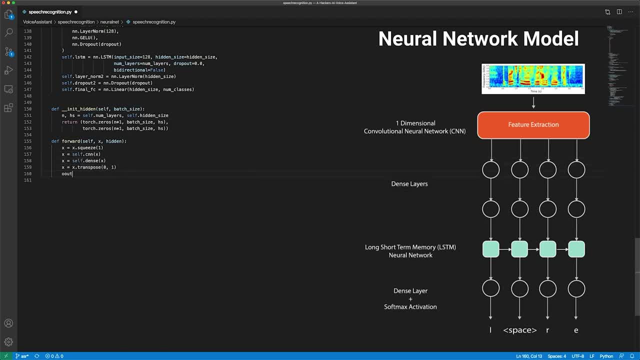 In deep learning, adding more layers can lead to better results, but since we want this to be a lightweight model, we stop at five layers. We have one CNN layer, one LSTM RNN layer and three dense layers. For the training script, we'll use PyTorch Lightning. 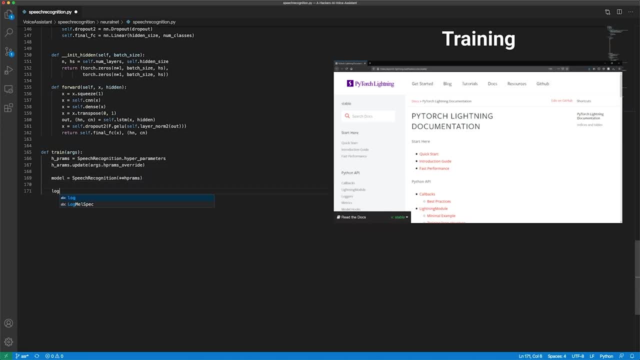 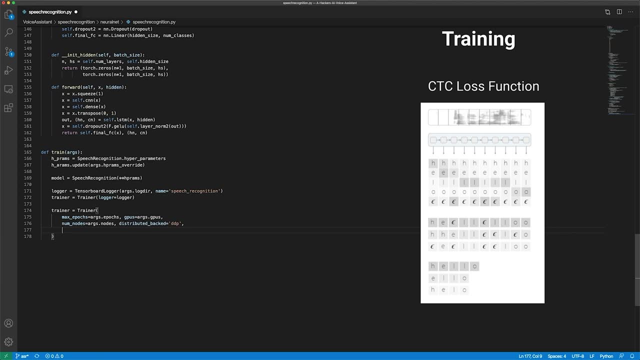 PyTorch Lightning is a library for PyTorch that decouples the science code from the engineering code. For the training objective I used CTC loss function, which makes it super easy to train speech recognition models. It can assign probabilities given an input. 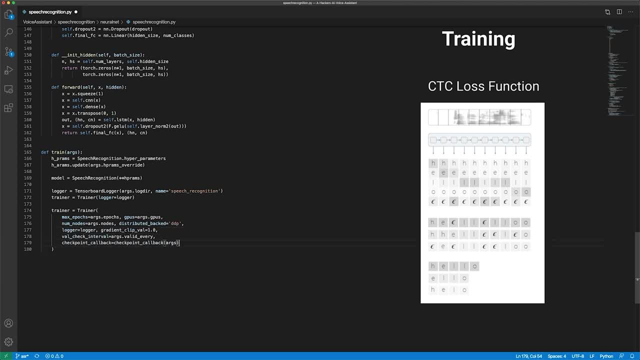 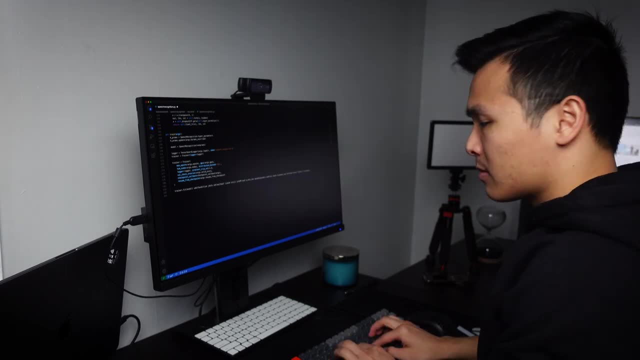 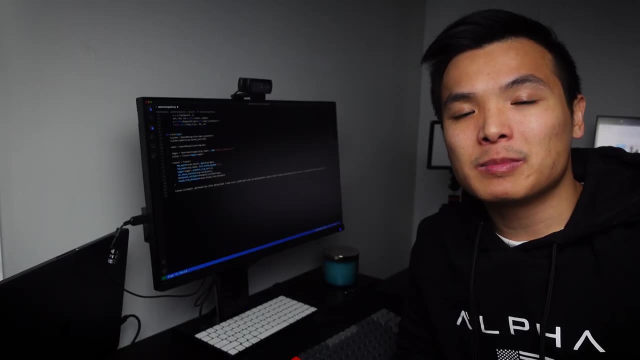 making it possible to just have your audio sample pair with their corresponding text labels, without needing to align these characters to every single frame of the audio. Oh hey, Just finishing up the rest of the code here. This code is open source, so if you want to see the full implementation details, 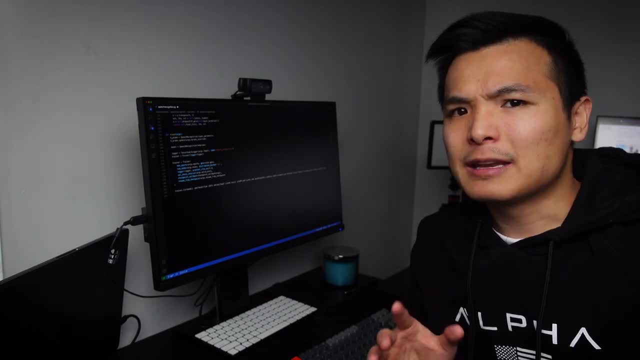 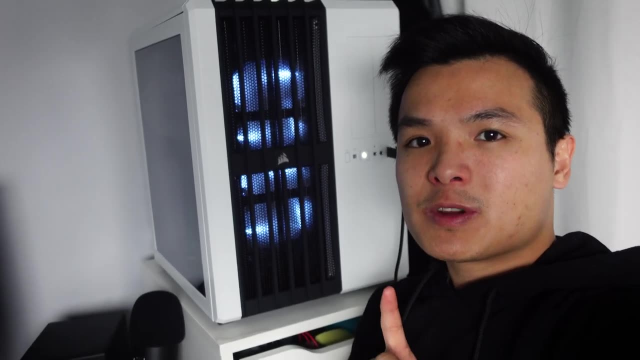 make sure you check out the GitHub repo in the description below. Now that we have the code, we need to start training. This is the perfect time to introduce my training rig, War Machine. War Machine is my personal deep learning rig I use to train models. 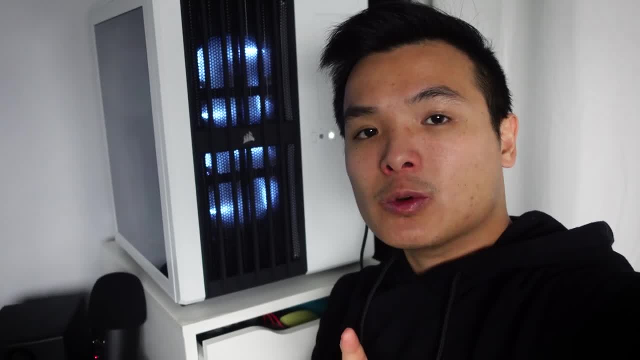 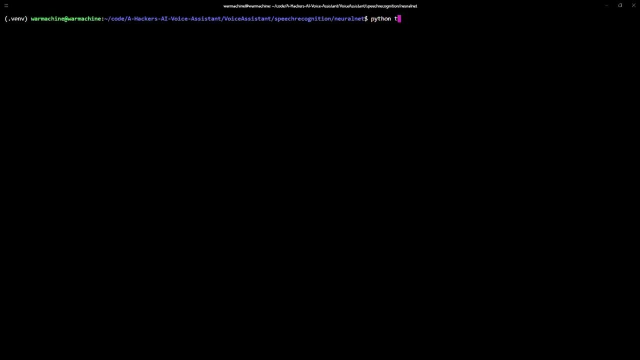 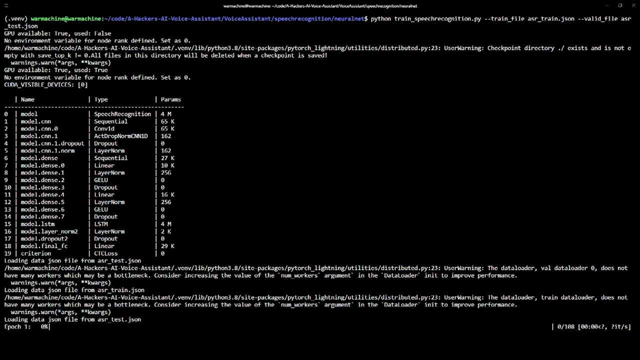 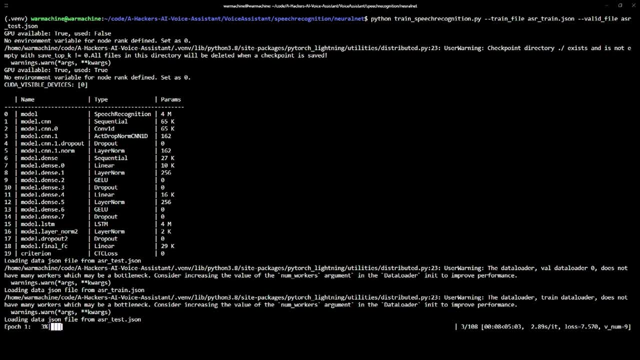 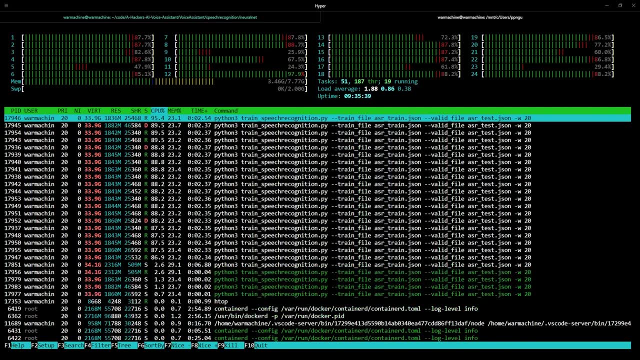 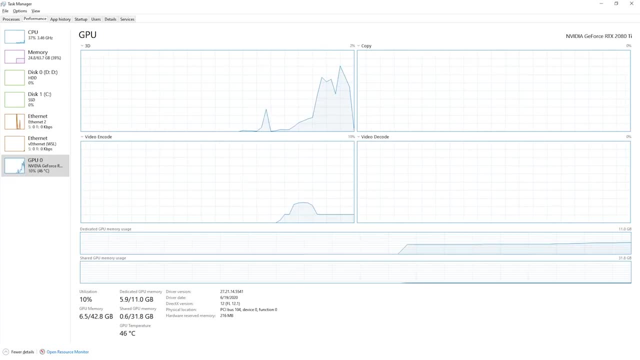 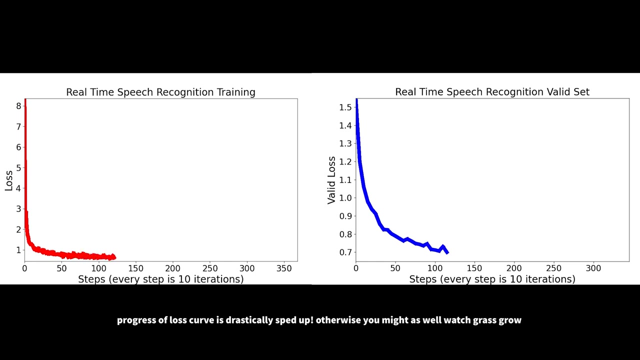 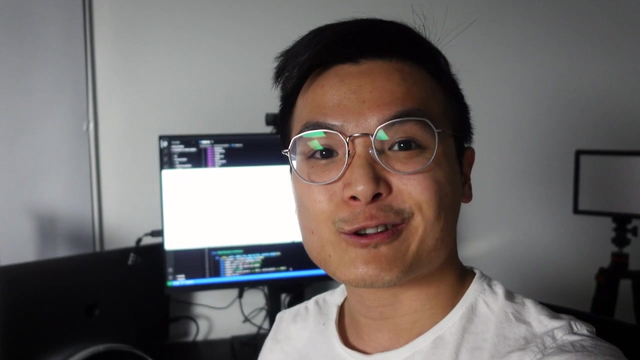 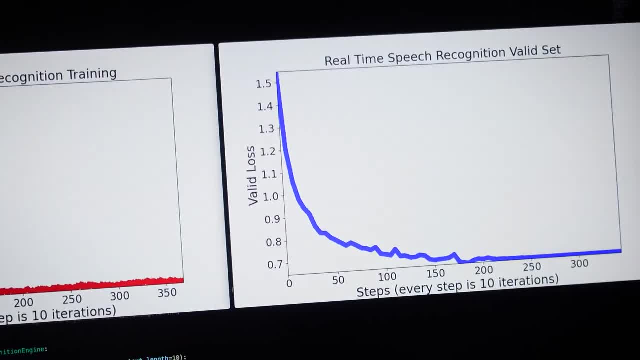 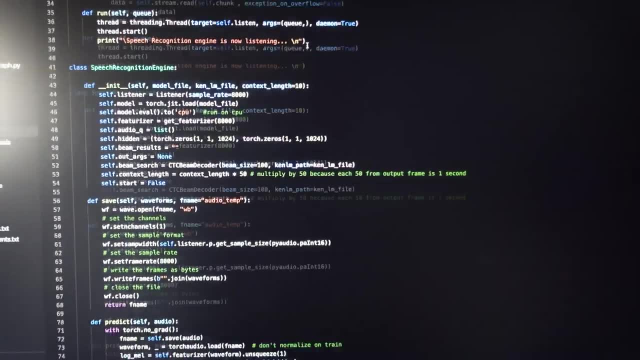 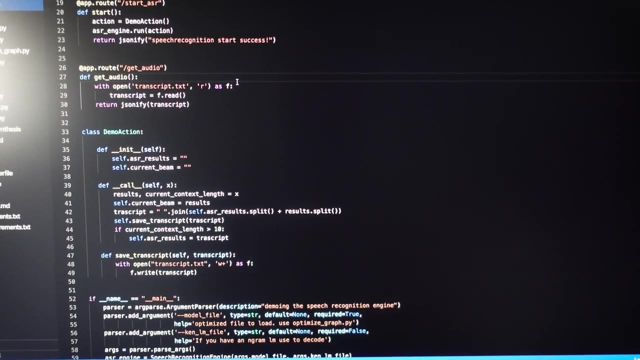 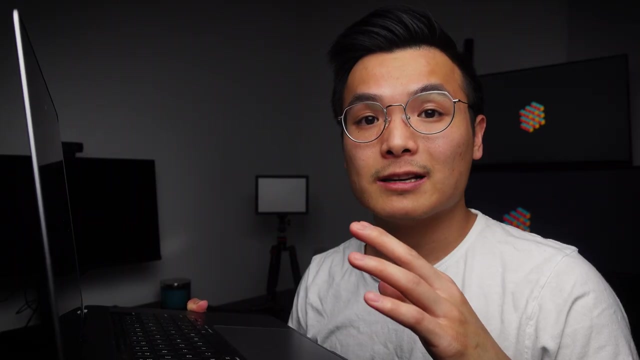 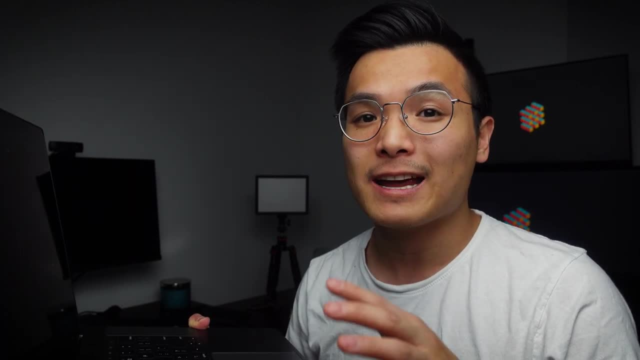 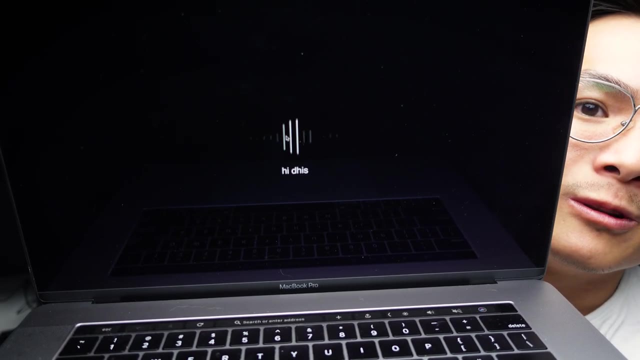 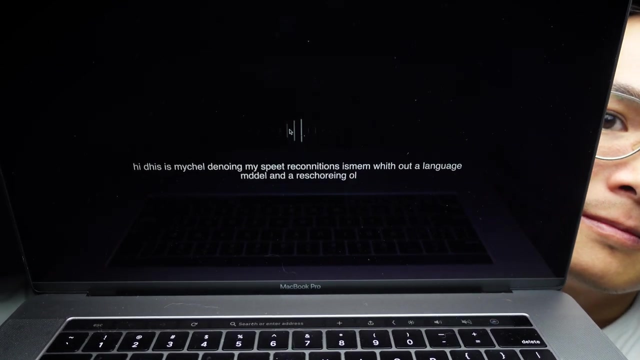 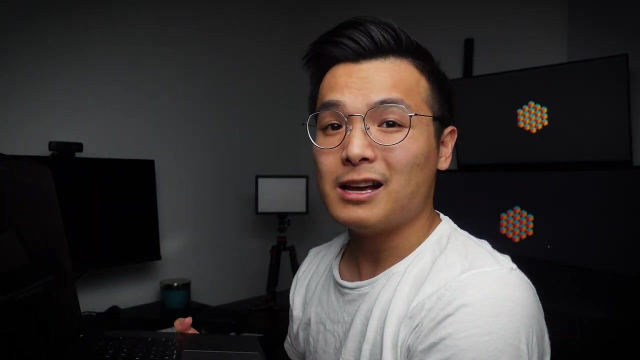 model and a rescoring algorithm. This is to showcase why it's important. Hi, this is Michael demoing my speech recognition system without a language model and a rescoring algorithm. As you can see, it's shit. It's not very good. Let me set up the second demo. 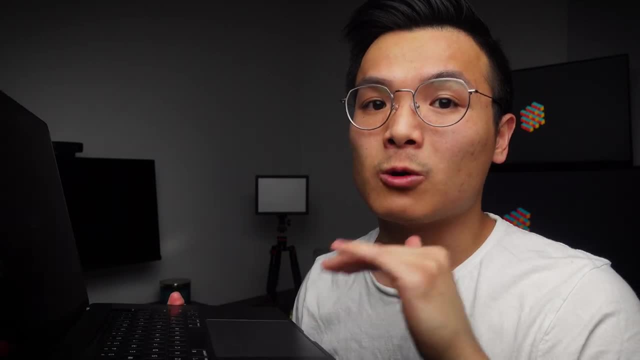 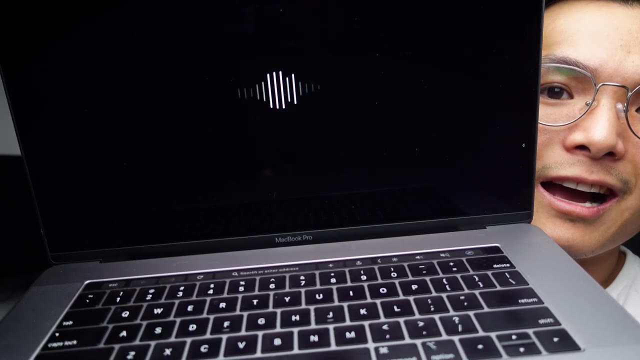 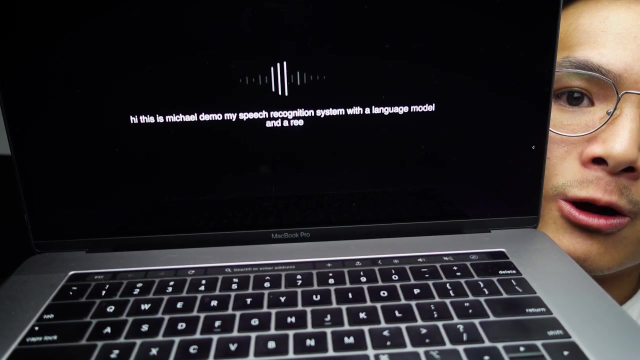 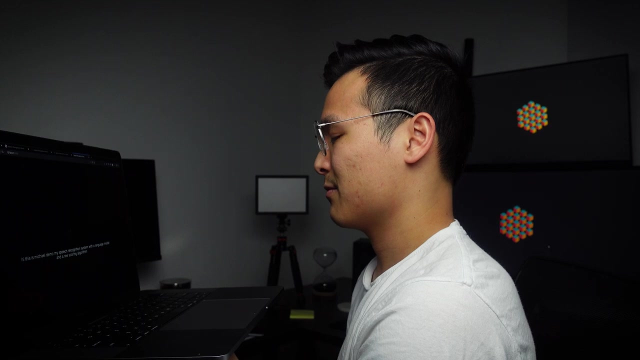 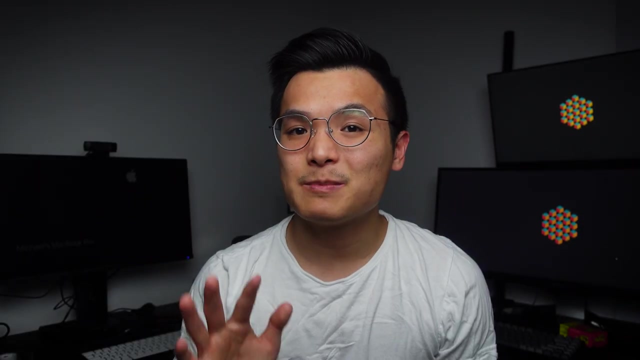 Okay, so this is the second demo with the language model and the rescoring algorithm. Hi, this is Michael demoing my speech recognition system with a language model and a rescoring algorithm. As you can see, it does a lot better, but it's not perfect. Okay, so the speech. 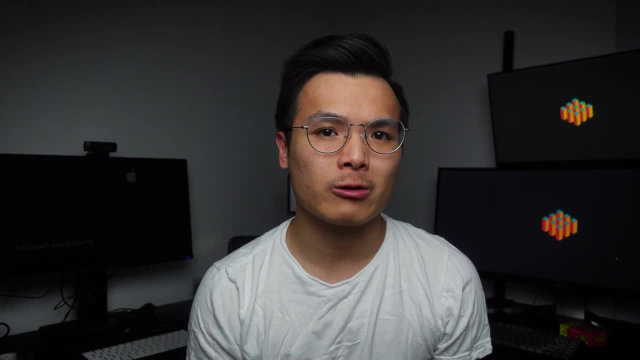 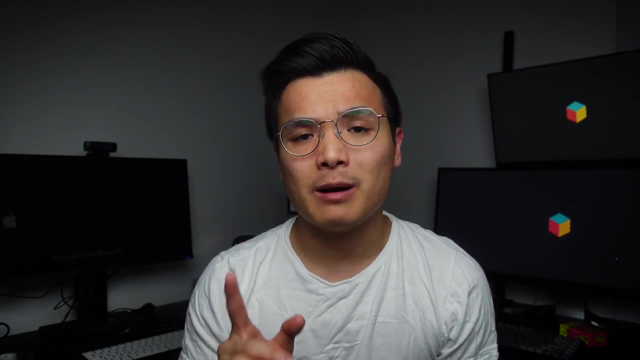 recognition system with the language model and a rescoring algorithm works pretty well with me. But let me reveal something I haven't mentioned yet. I collected about an hour of my speech and trained it to how to do the speech recognition system, and that I've seen before. 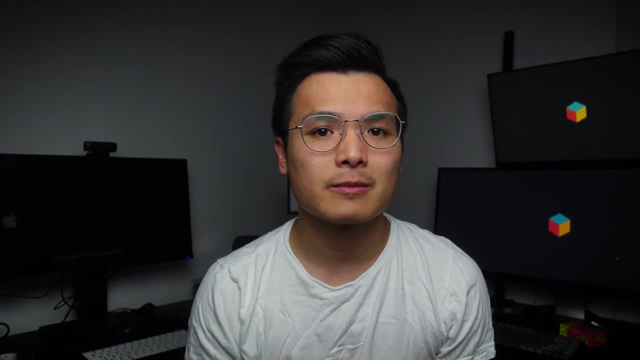 with the common voice data set, which is about a thousand hours. One thing I forgot to mention when filming this clip was that I also upsampled the one hour recording of myself to about 50 hours so it can be more representative in the entire training data. 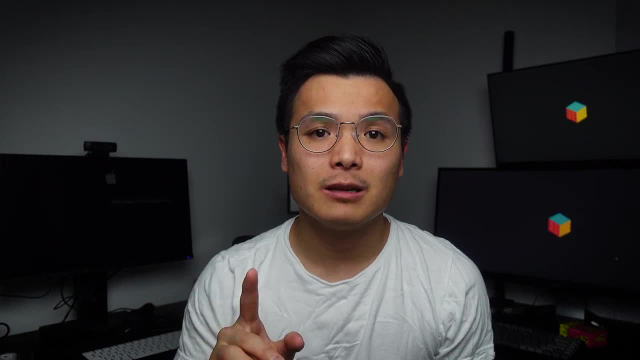 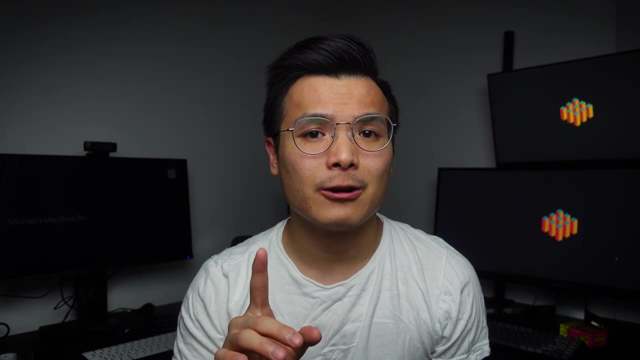 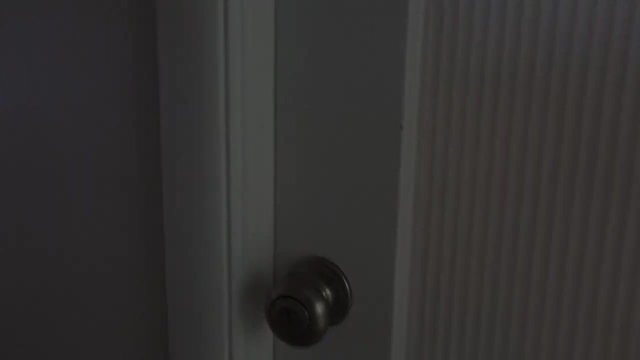 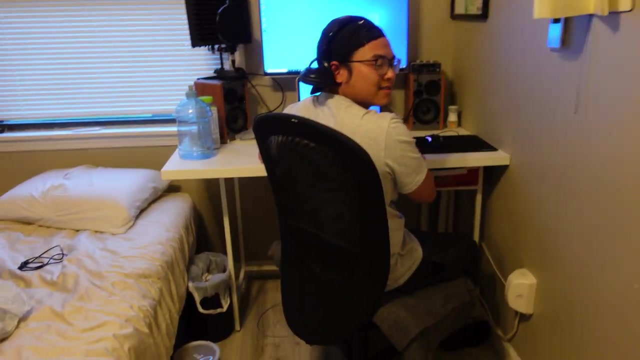 set, Okay, play. So there is a possibility that that extra hour of my voice has biased the algorithm to work really well with me. So to test that theory, I want to try the speech recognition system with other people. Hello, Yes, this is my brother Long Long. I need you to test this out for me real quick. 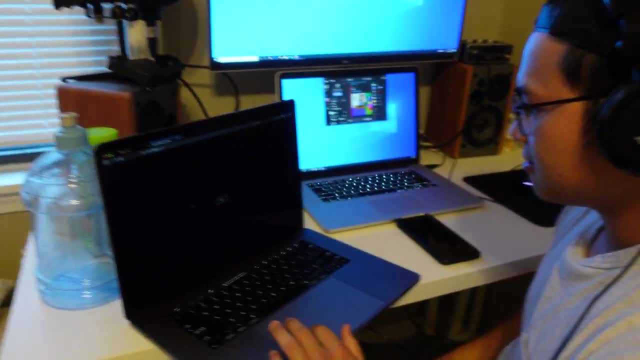 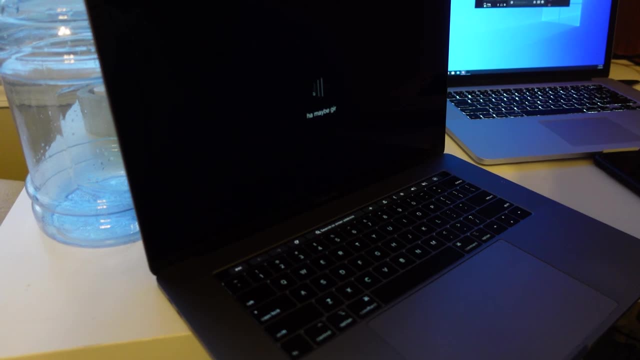 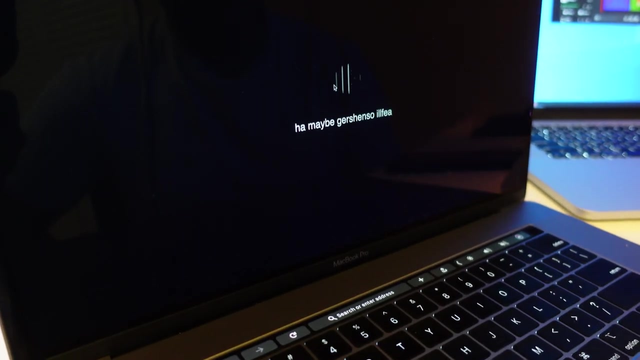 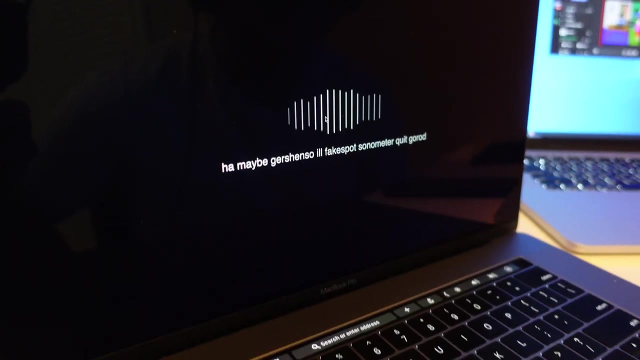 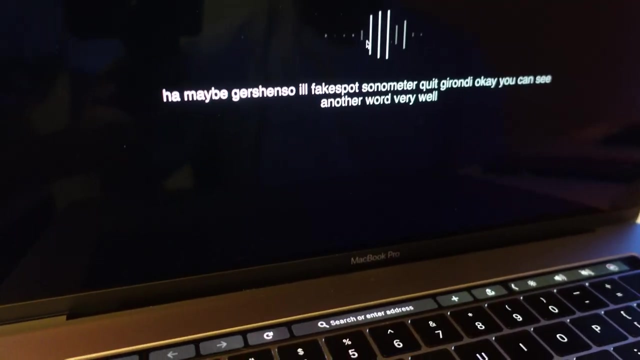 All right, Just press that start button and say whatever you want. Hi, baby girl, Say something else, You look fine. Okay, say some more stuff. Hey, you better quit f***ing around. Okay, as you can see, it doesn't work very well on his voice, but when I start talking, 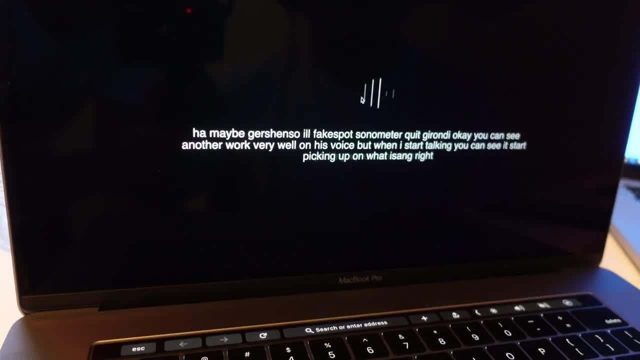 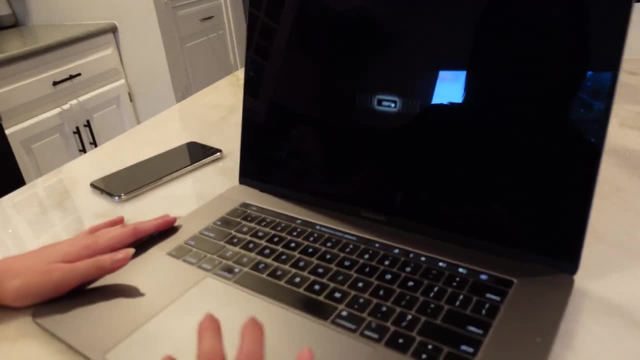 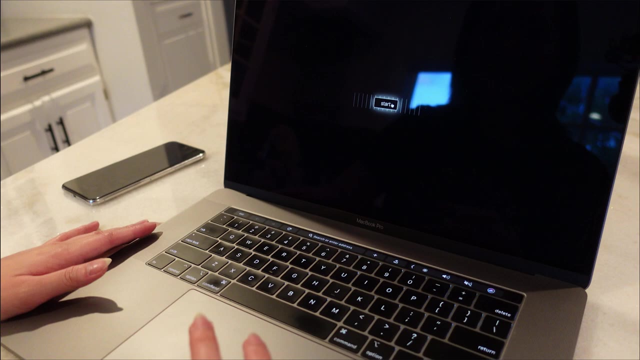 you can see it start picking up on what I'm saying, right? Oh, dang, that's cool. Okay, thank you. Okay, so our next guest is big on privacy, So we'll just skip the introductions and go straight into the demo And play. 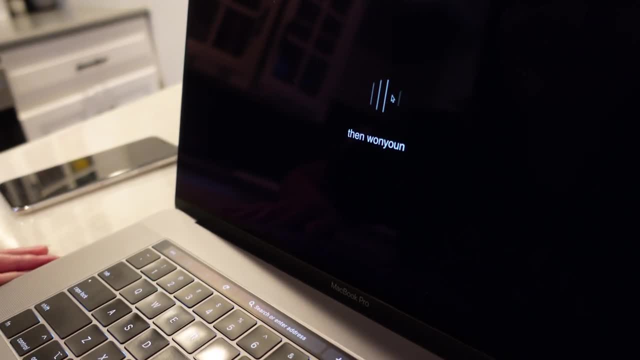 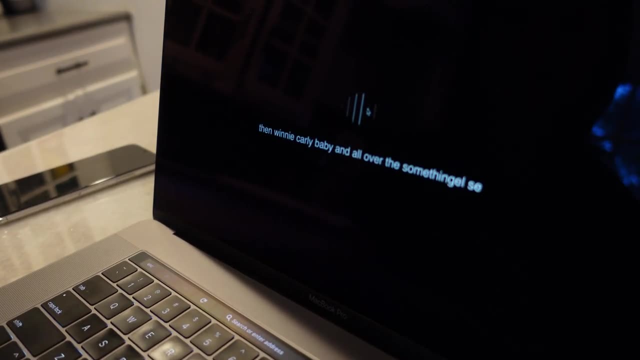 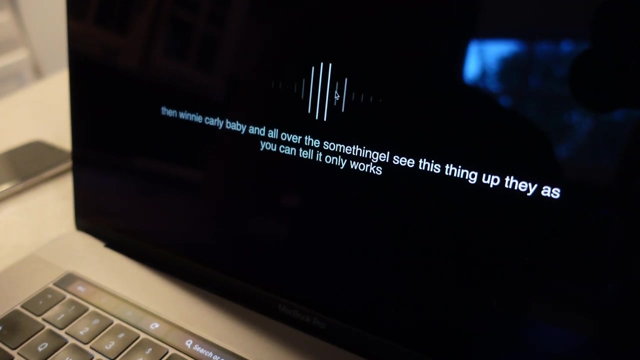 Say anything you want. I love Charlie, baby and Oliver. Say something else. This thing sucks. Okay, as you can tell, it only works well for me. again, It doesn't work very well for her, so she thinks it sucks. 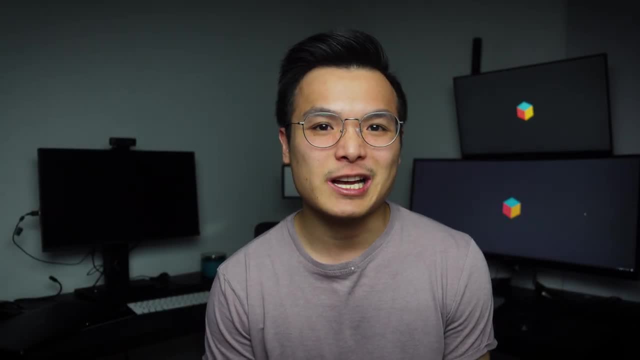 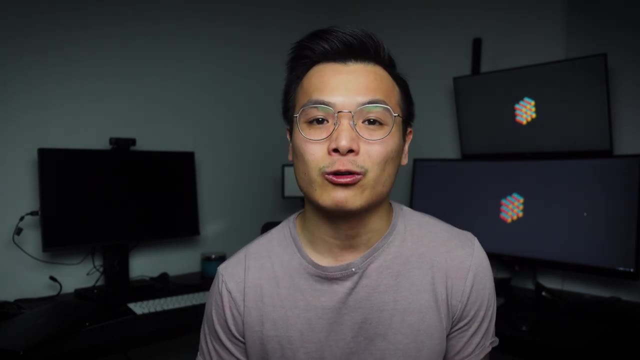 All right. so, as you can tell from my guest's reaction, a speech recognition system is not that great. at least on them Works really well for me. That's because I biased the algorithm by adding my own data. All of this was expected though DeSpeech2, a very famous speech recognition. 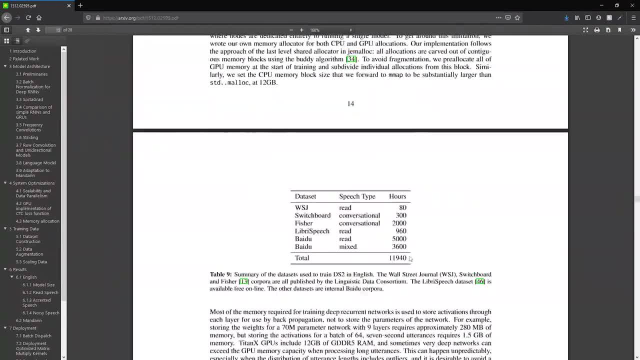 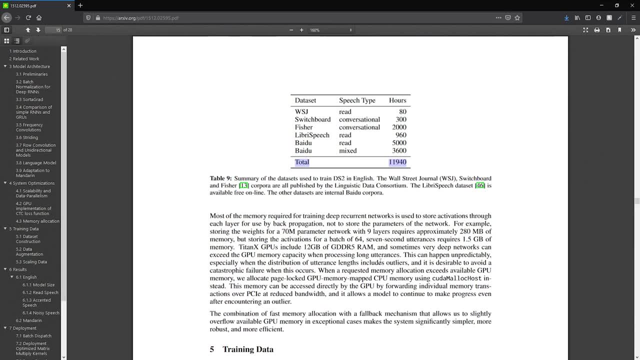 paper from Baidu claimed that you need about 11,000 hours of audio data to have an effective speech recognition system, and we used: like what? 1,000 hours or so. Their model also has 70 million parameters.